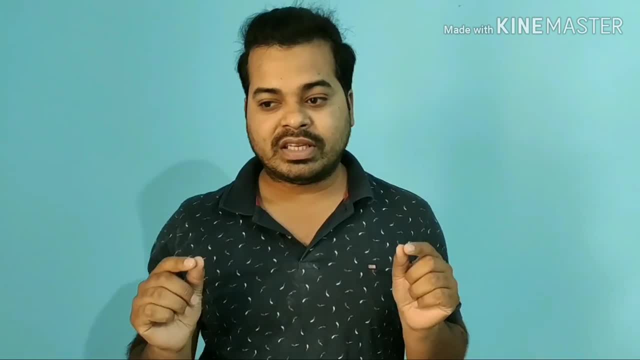 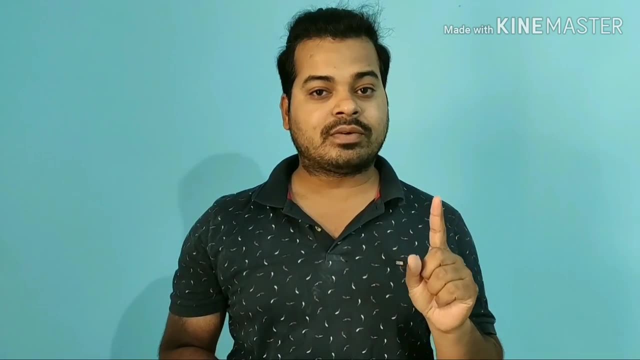 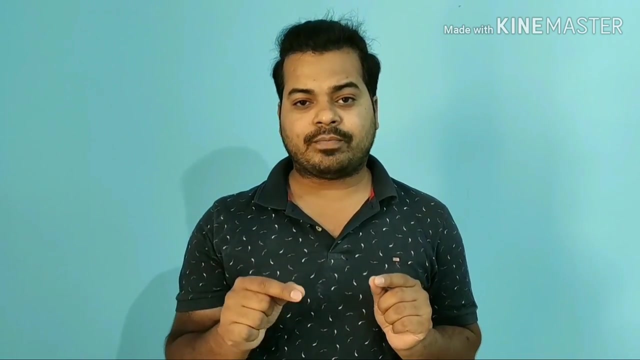 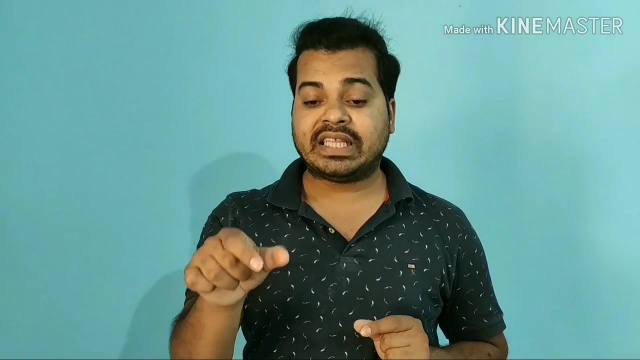 development lifecycle. the stages we have are- listen clearly, guys. the first stage is call as requirement collection. first stage is called as requirement collection. that means now the portion arises. who do the requirement of extra requirement collection is done by product analyst. product analyst is the person who will be in the product based companies and business analysis. a voice. 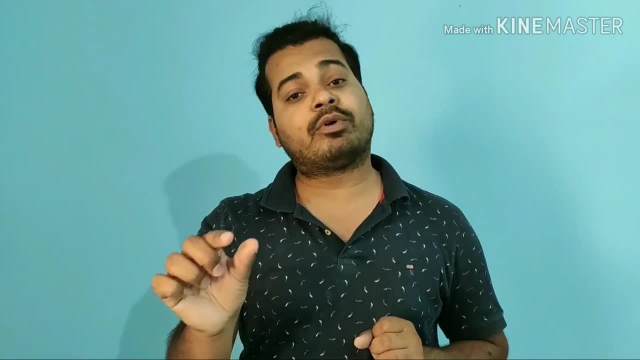 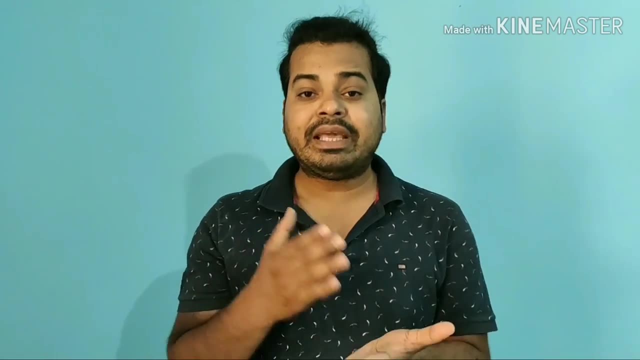 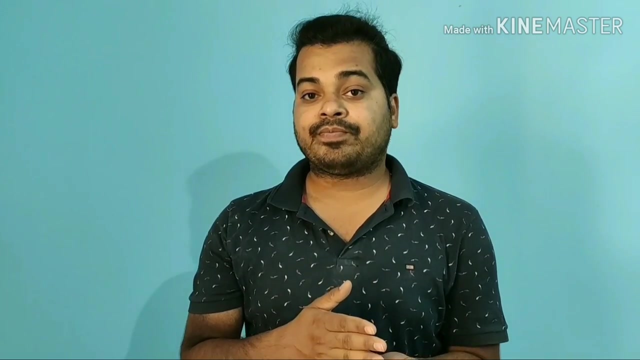 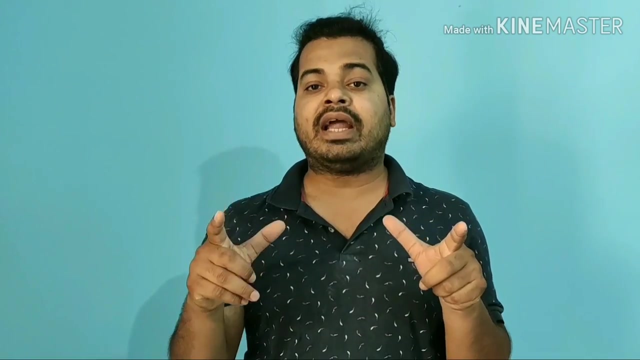 we will do the requirement action companies. okay, so BA business analyst. he will go to the customer case, he will collect the requirement in the business language. he will come back to the company, convert everything he has understood in the business language to technical things and he gonna explain it to the technical team. technical team. 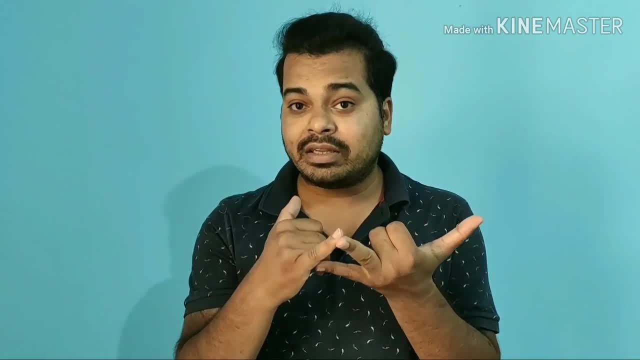 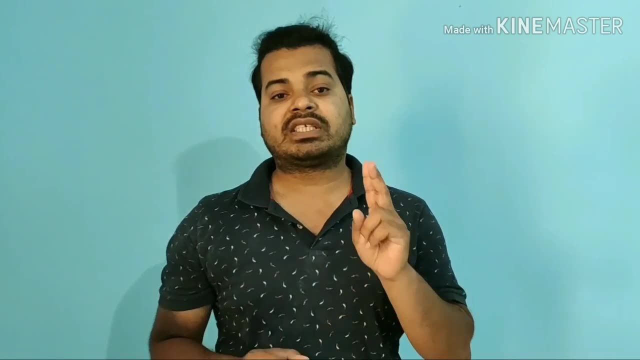 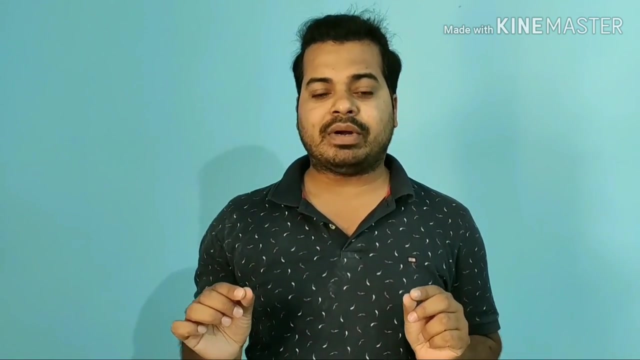 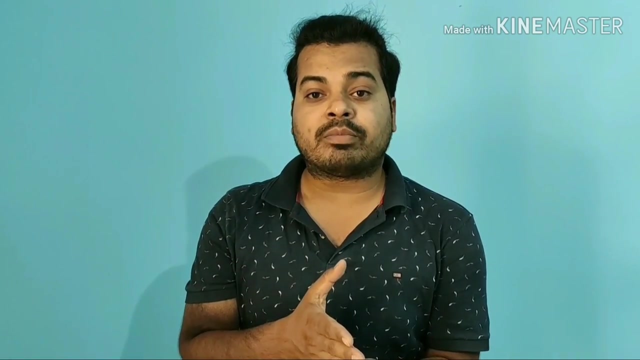 consisting of architects, developers, product head, that is, product managers- and QA- QA engineers. this is, this was the first step. the second stage of SDLC is called as feasibility study. now, feasibility study is nothing, but in this stage they define whether to take up the project, if they are going to take up the 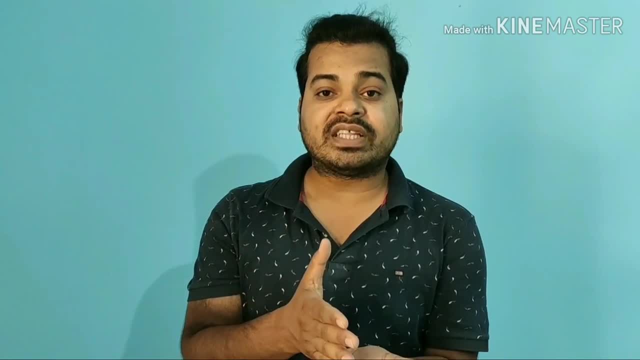 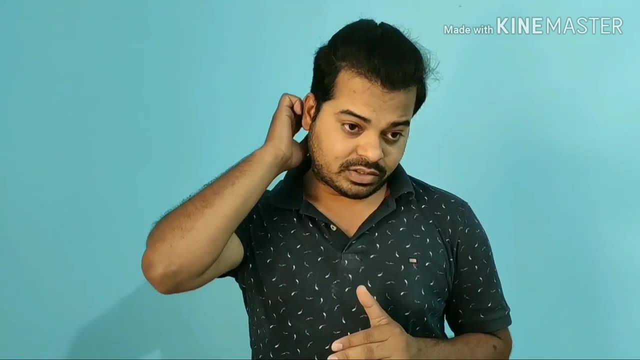 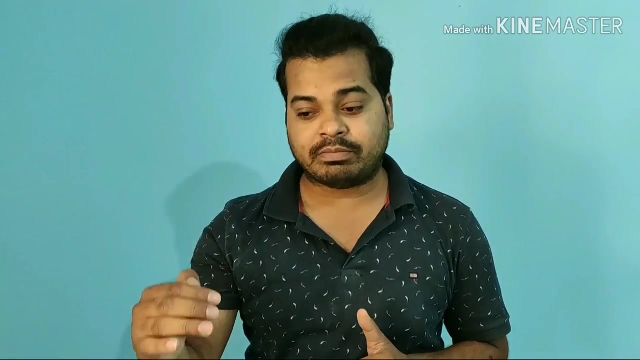 project. are they going to get any profit or not? so this is the stage where they decide whether to take up the project or not, this stage consisting of different teams. the first stage is feasibility study, so this is the stage where they take up the project and when the two are lining up: the first, the first one, the 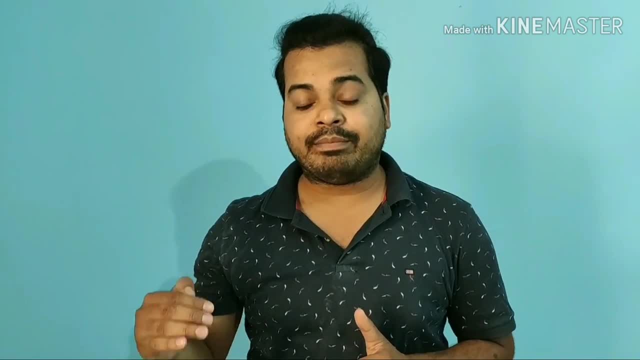 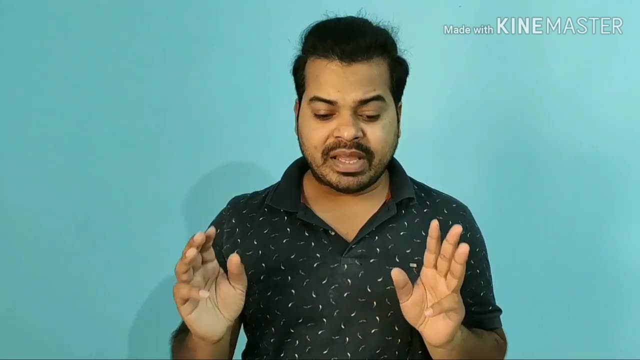 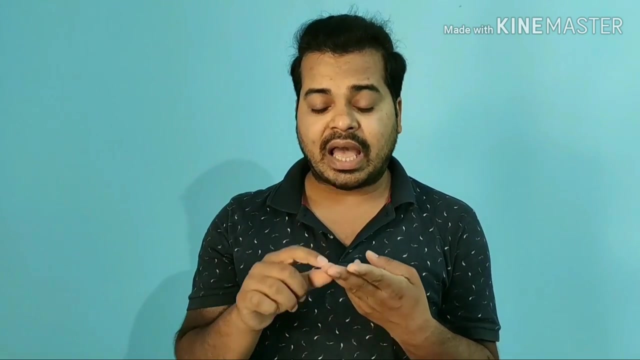 first person is called as Product Hand or Product Manager. the second is finance team, HR team, architects and BA Business. these are the people who decide whether to так up the project or not. they may talk about three things: whether they have enough resources to take up the 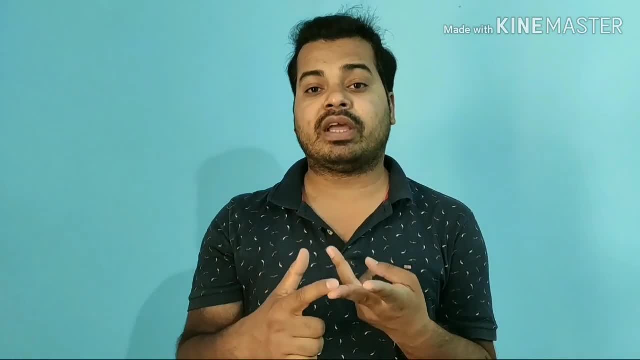 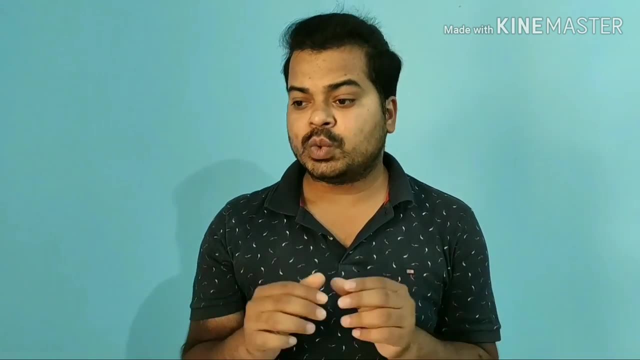 project. when I talk about resources, I meet whether they have proper engineers, developers and QA to take up the project, whether they have enough resources to up the project or not. do they have? second is: do they have proper lab setups or not? do they have proper lab setups or not? i mean, if they take up the project, lab setup is required. are they having? 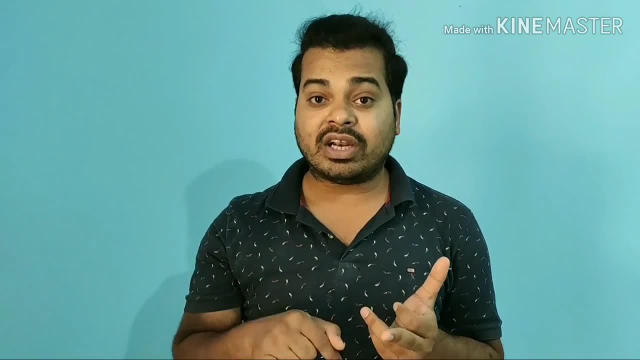 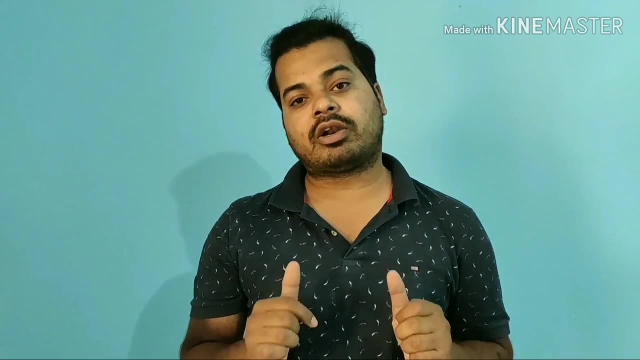 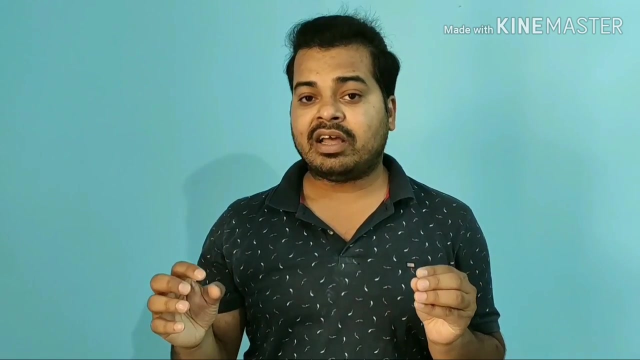 it. and the third is which? are they having the technology to take up the project or not? so they decide on these three mainly things to decide whether to take up the project or not. now i'm going to talk about the role of product manager. he is the person who will take the data from. 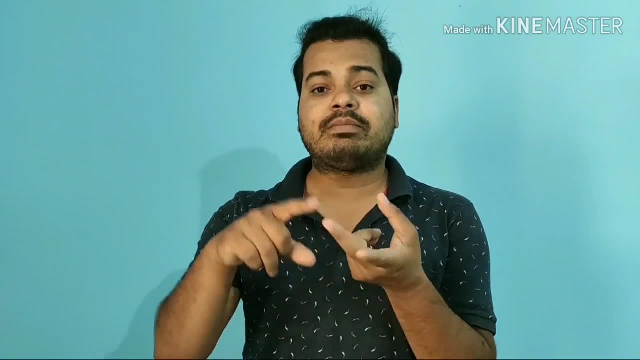 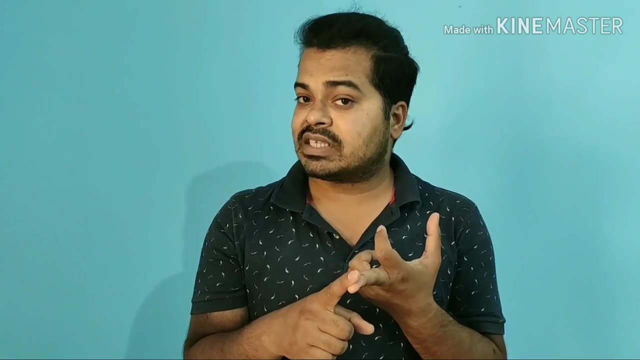 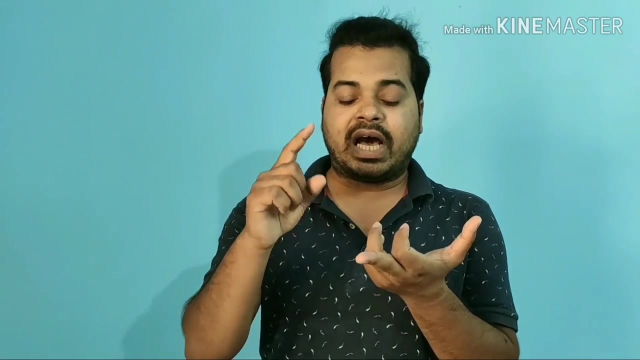 business analyst, architect, finance team and hr team and he is the person who will decide whether to take up the project or not. how ba ba is the person who will collect the requirement. as i have already said, his role is to collect the requirement. he is going to uh requirement and architect is a. 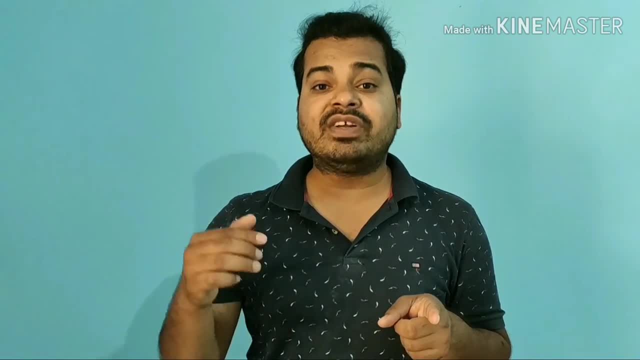 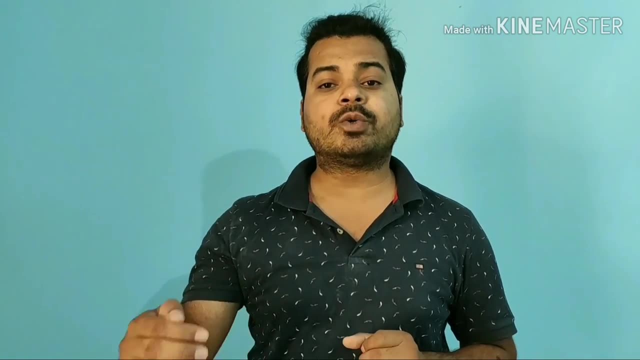 person who will think from the technical point of view that means which technology to to take up the project financing. they will think from the money point of view: if they are going to take the project, are they going to get any profit or not? if they invest this much of money, are they? 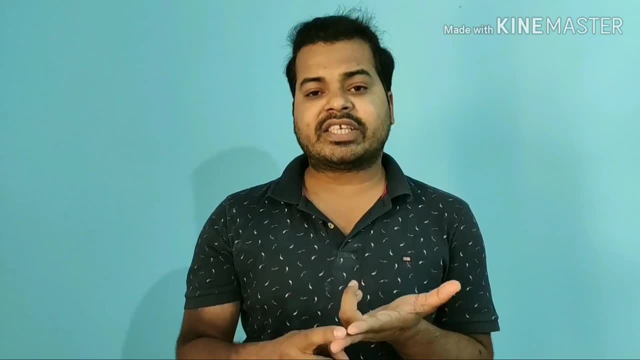 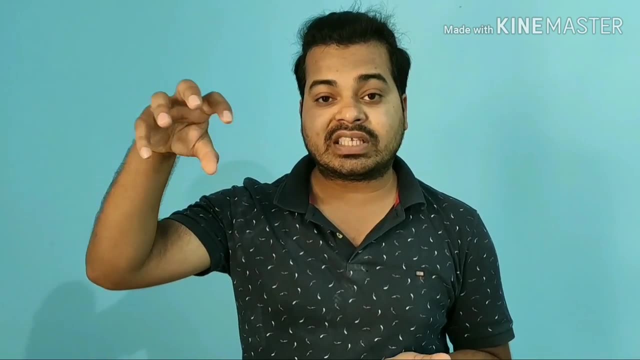 going to return anything? are they going to get profit? so an hr team, hr team, technical team- is the people who will tell that they require this many engineers in the project. so it is the job of the hr team to hire those people. he will collect product hand. that is product manager. he will. 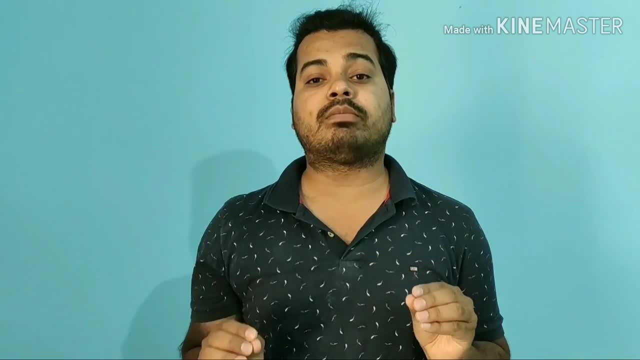 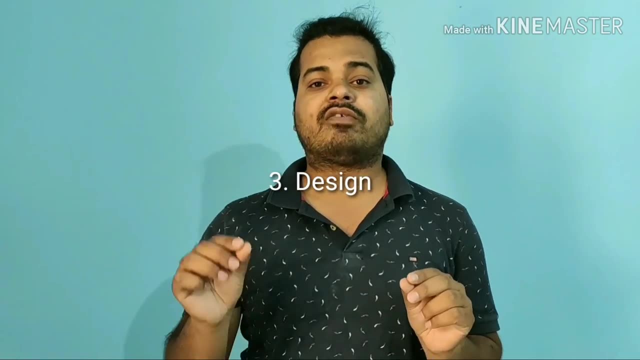 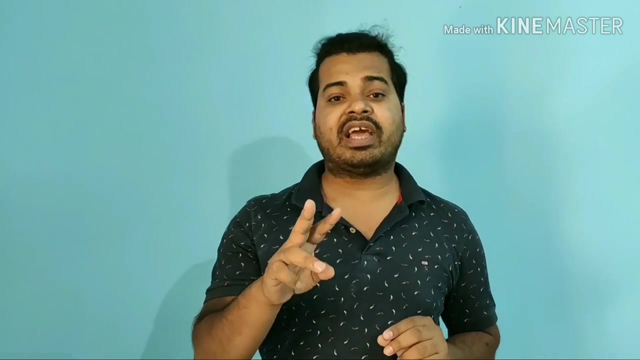 take the data from everyone and he will decide value who take up the project or not. this is a feasibility study. i have explained in a very easy language. third, third stage of software development life cycle is called as design. design is mainly done by architect. in design we have two things. one is high level design, another one is low level. 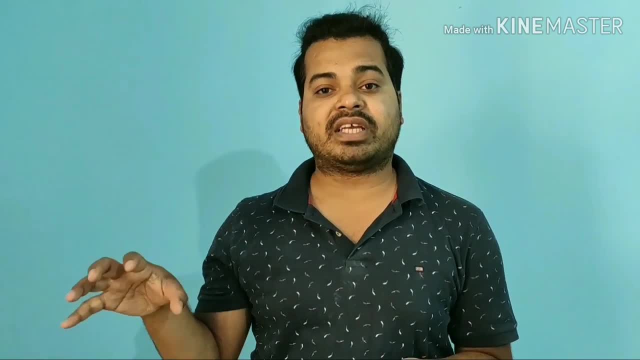 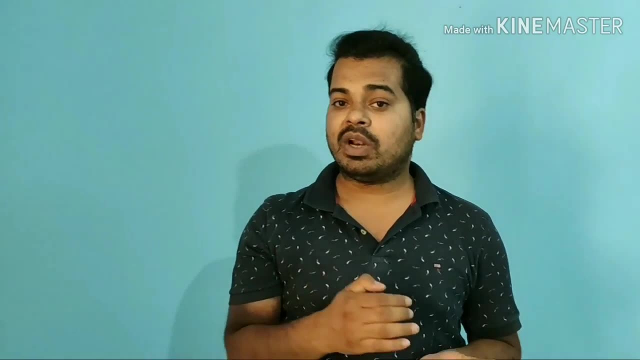 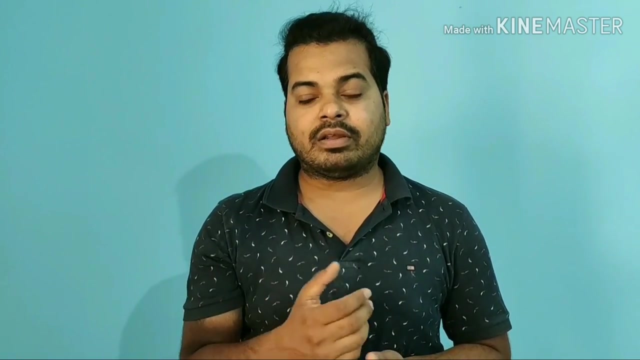 design. high level design is designing the architecture of the application. how the application look will look like. that is called high level design. if i talk about the low level design, each and every modules will look like. that is called as low level design. so i hope i mean- if i'm 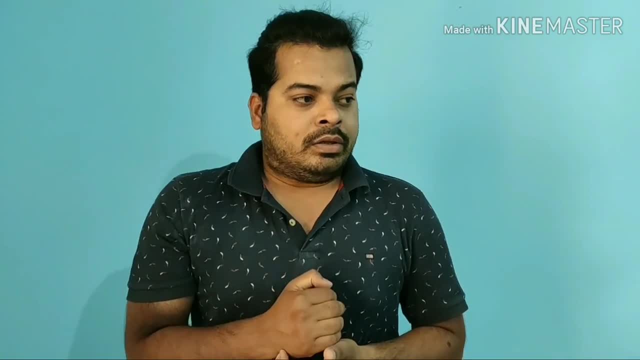 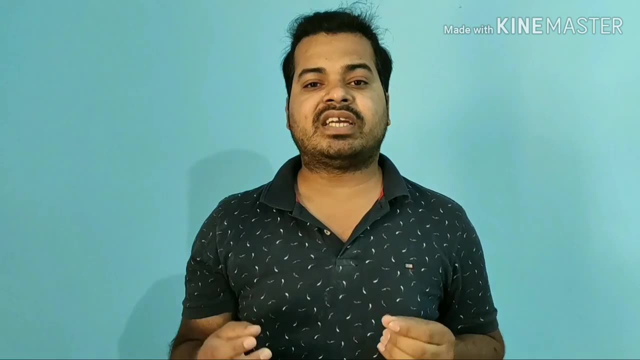 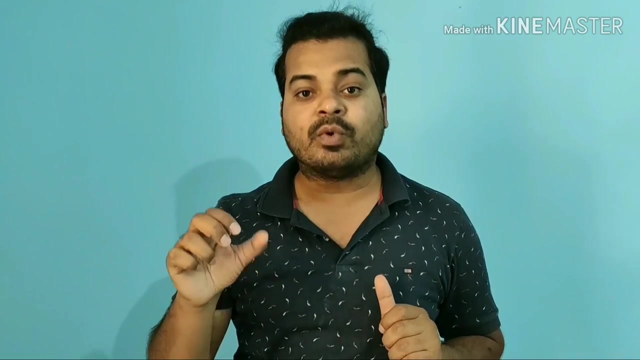 going to give you example. you guys will understand in a very better way. let's take example that i have. i have bought a site. i have bought a site. now i have decided that i am going to construct, in that i am going to construct one room, one hall, one kitchen, two washrooms, one lawn, one parking area. 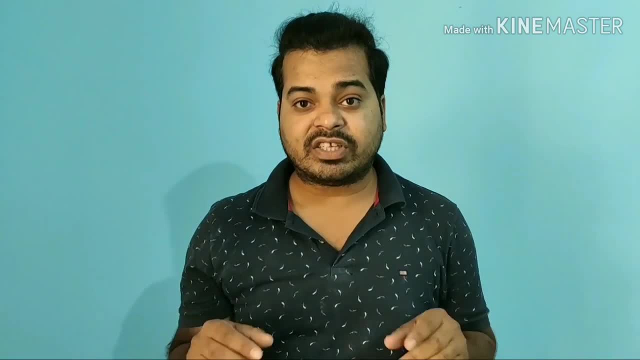 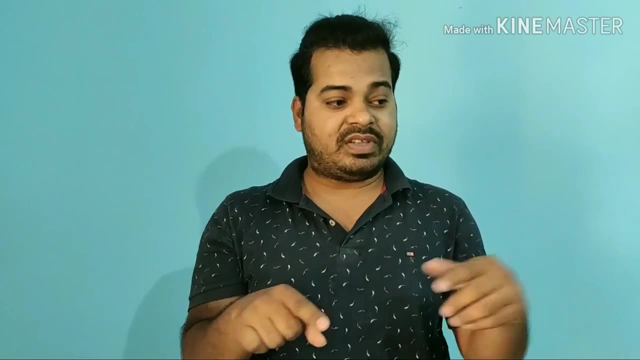 these are things i'm gonna make in my site, which i have bought. that is called this high level design. now, what is low level design? suppose my site is like this: this is the entrance. i will be having my first room here with that attached washroom, will be there with that attached living room. 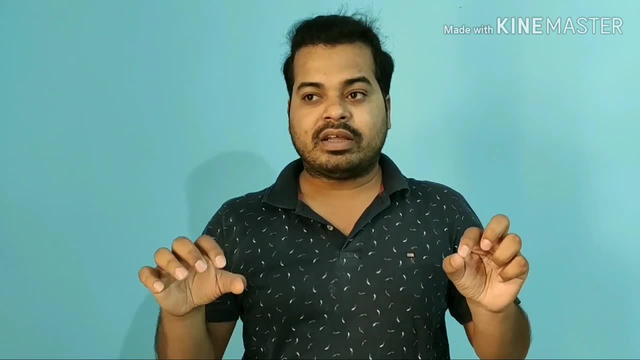 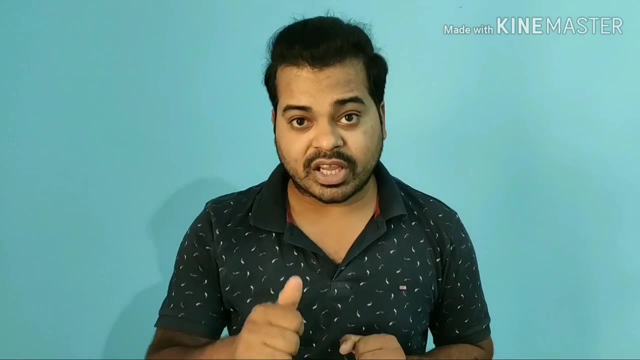 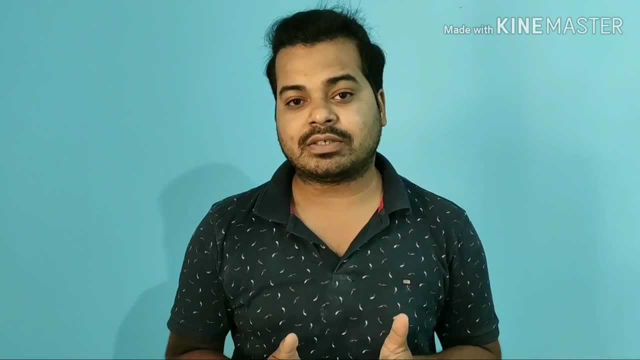 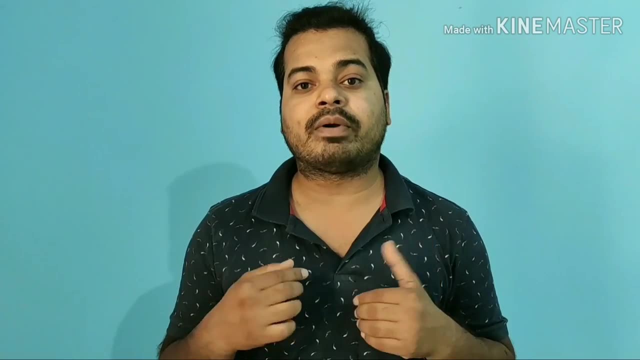 what's up is having an option called as select a contact. i send a message. they also have a option of attachment that is called as high level design. so i'm going to talk about low level design. if i click on attachment, it is having multiple options in it. let's say it is having an option. 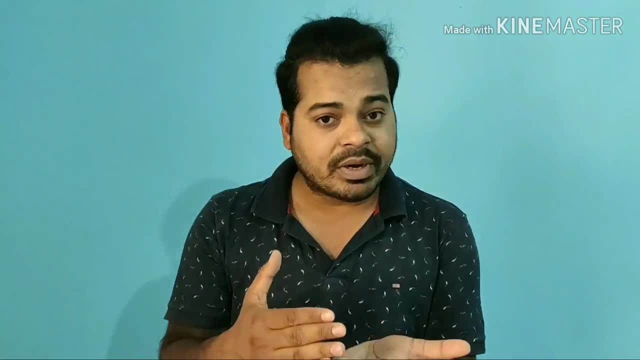 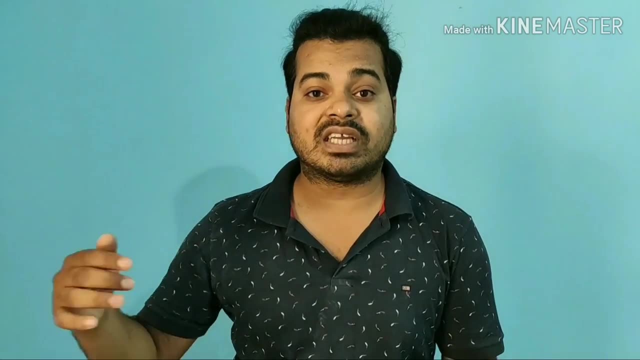 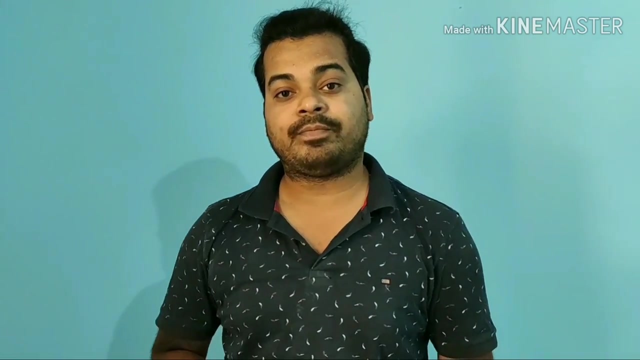 of selecting an image, video, document location files. they have multiple options to select. so that is called low level design. i'm talking in depth that talking if. if i'm talking about any software in depth, that is for this low level design. i'm going to give you one more example, talking about uh gmail. gmail is having an option of 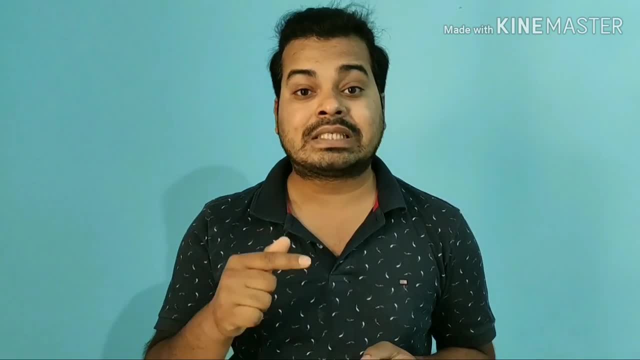 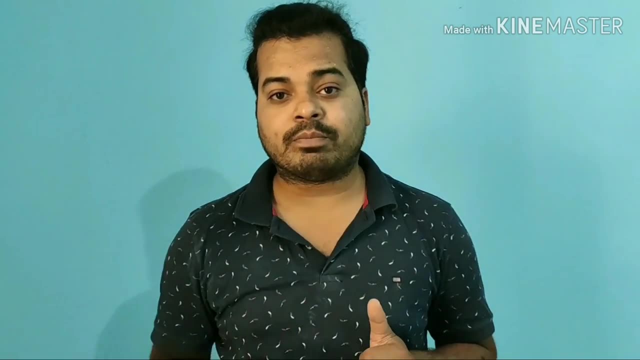 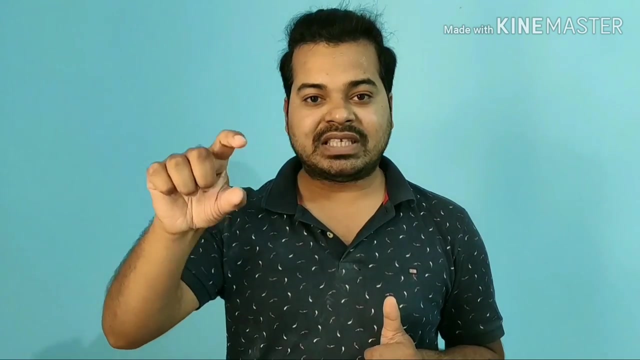 composing a mail: sent mail, outbox, spam, logout, login. that is for this high level design. now, what is low level design? if i'm gonna do a compose mail, it will be having an option called as two to whom i'm sending from. that will be my mail id: bc, bcc. 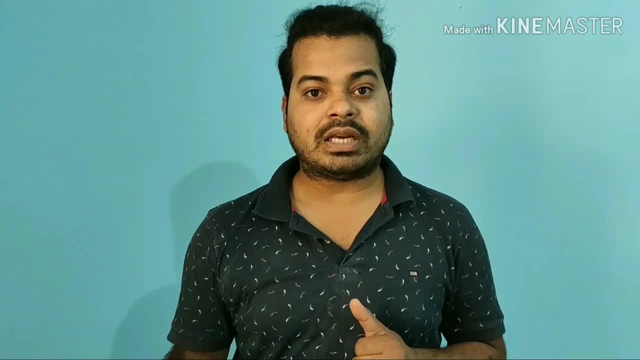 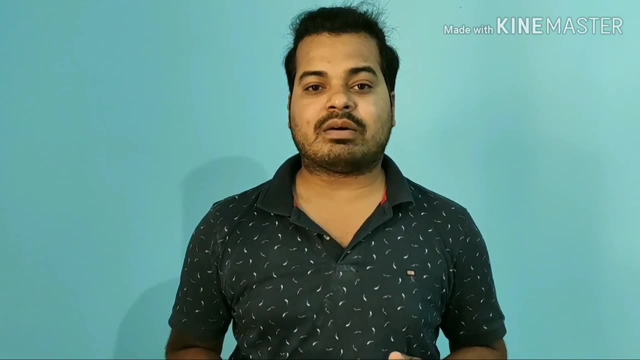 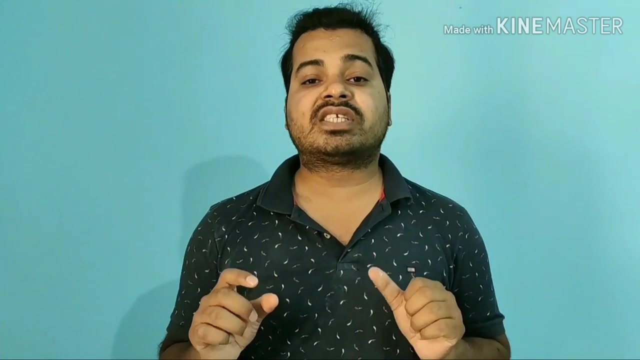 subject: body attachment. send button, cancel button. signature. that is called as low level design. i hope it is very understandable, right? so once the design phase is completed, the fourth stage in software development lifecycle says that coding, coding has to be done. developer will start writing the code by seeing the low level design and the requirement and always remember. 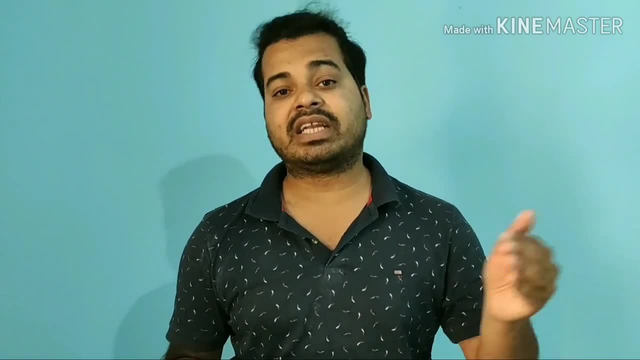 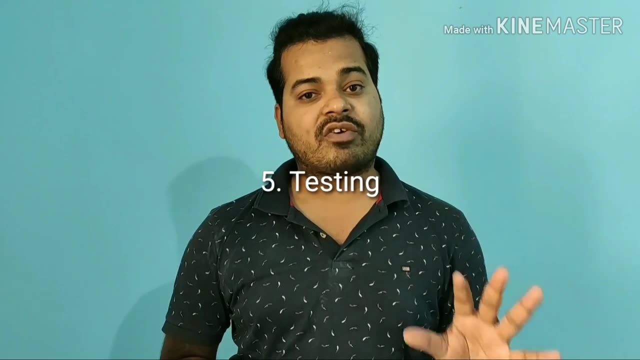 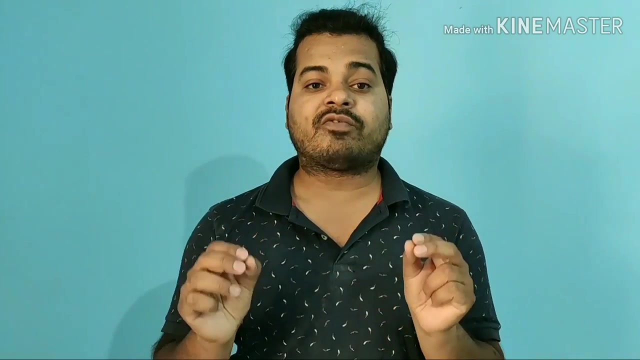 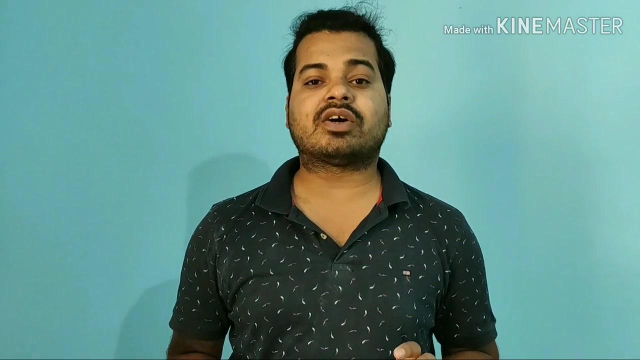 business analyst. he is the bridge between the customer and the developers. so once after the coding is done, the fifth stage of software development life cycle is called as testing, which we will be doing it. once the testing is done, software is working perfectly fine, we are going to release it. that comes the sixth stage. the sixth stage is called as installation, and 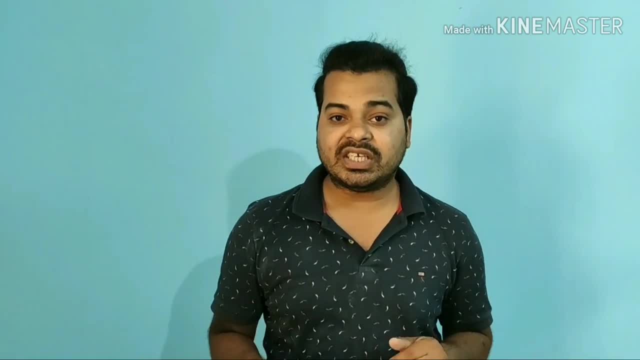 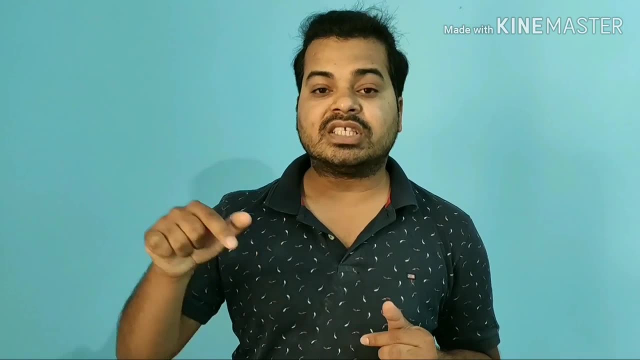 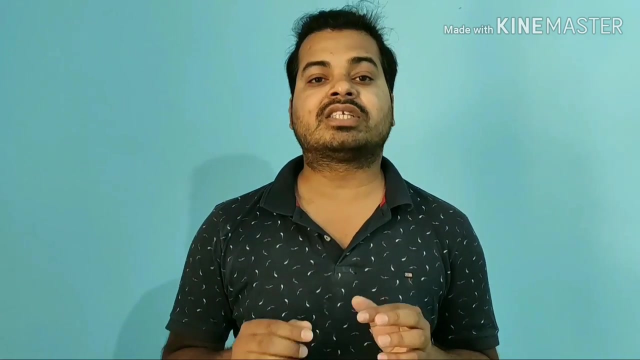 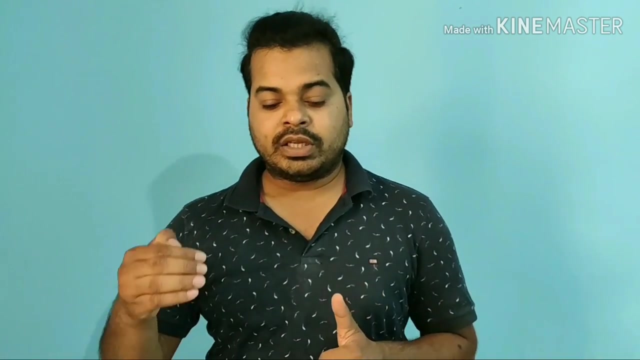 implementation, our site engineers, site engineers, field engineers. they will go to the customer's place, install the software, make it ready so that customer can start their running their business with the help of the software. that is called installation, installation or implementation, clear, great. coming to the seventh stage, that is called as maintenance. 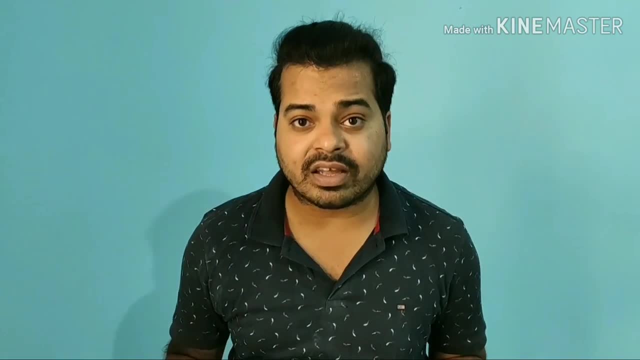 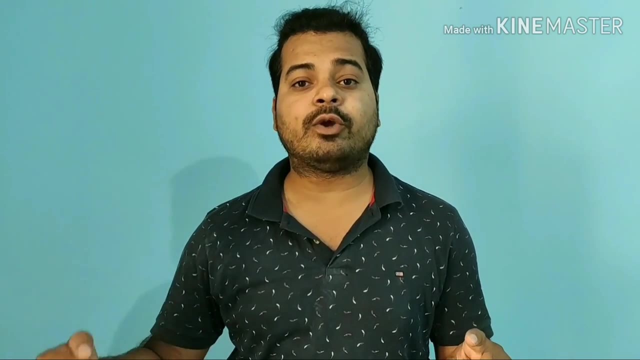 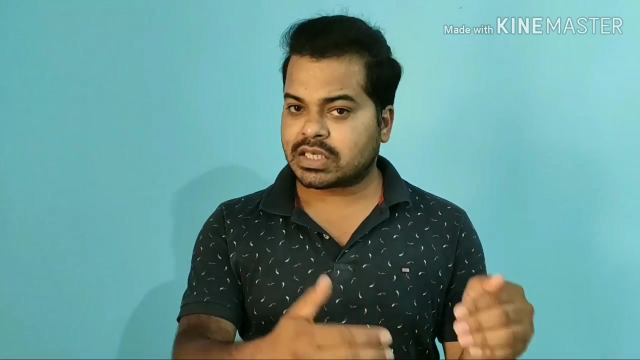 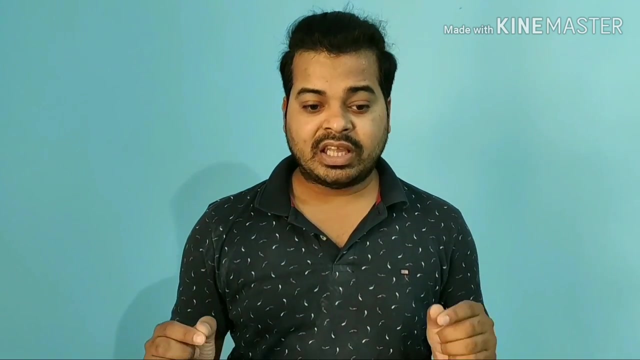 phase. the last stage of software development life cycle is called as maintenance phase. maintenance is done by developer and qa. now i'm going to tell you what do you mean by maintenance phase. once we have given the software to the customer, there will be a service level agreement for six months or one year. that means while using the 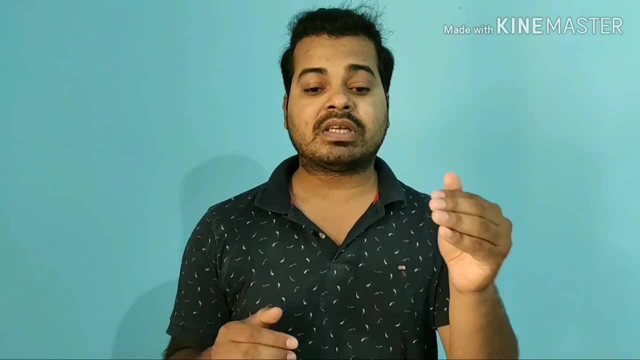 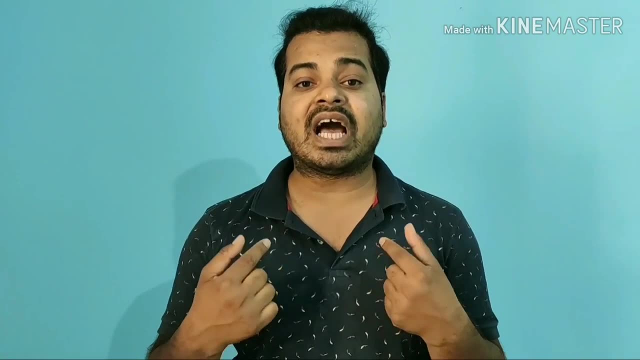 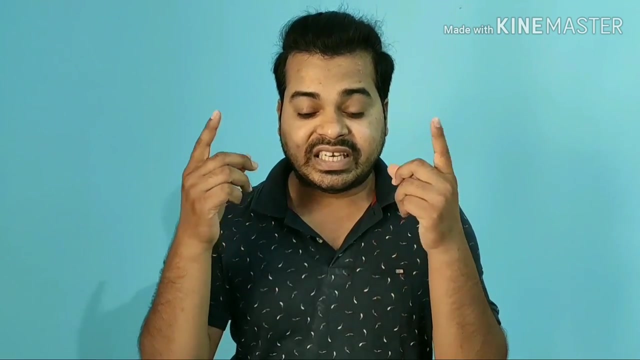 software if customer is facing any defect, if customer is facing any problem and you want to change it, it will be written in the service level agreement that we will be providing our maintenance for a period of six months or one year. so we will be developing it, developer will be developing it. 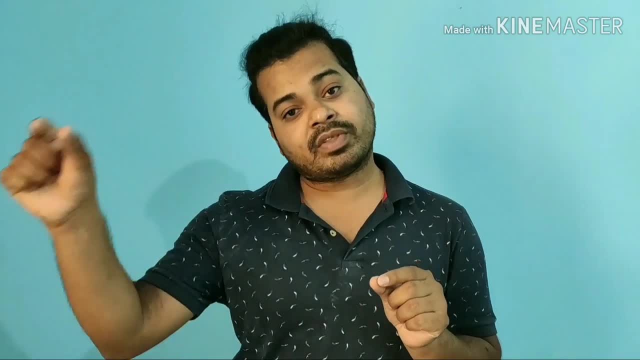 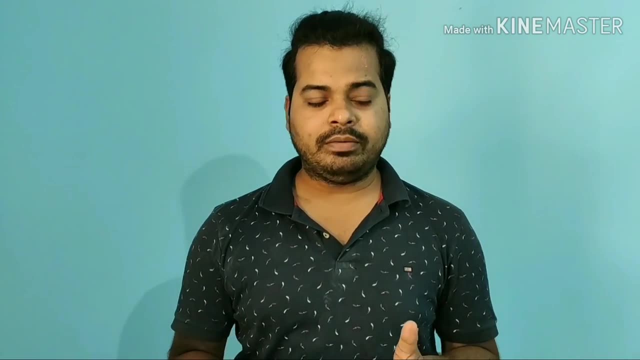 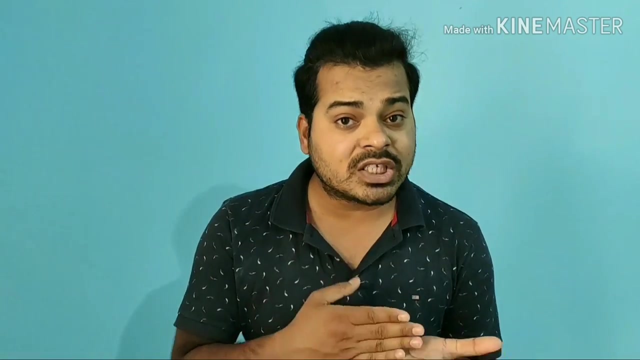 test engineers will test it and we will give a new software to the customer over a period of service level agreement- how many period it is having six months or one year- done once after service level agreement is over if customer wants to do any modification in the software. 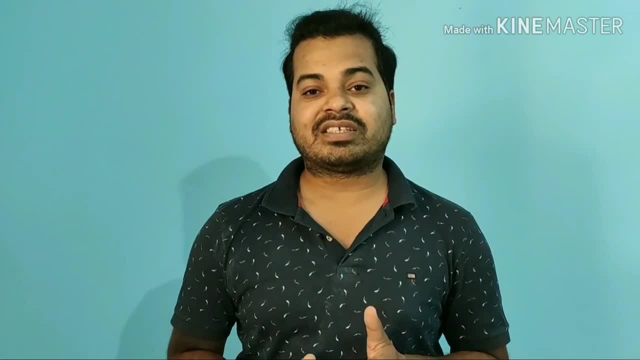 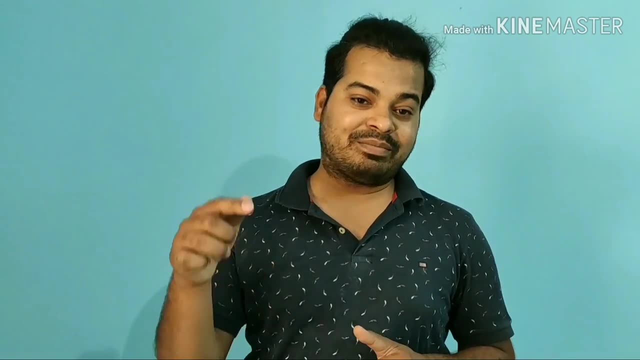 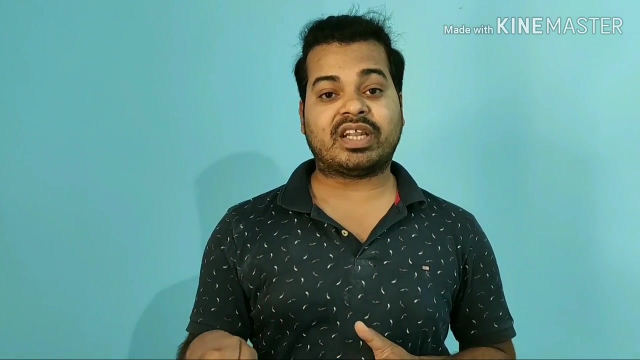 they have to pay it and get it, so that is called a software development life cycle. i hope it is very clear. i have explained in a very easy language. if you have any question, please reach out to me. i have added my gmail id in the link description. i have my quora profile in the link description. i 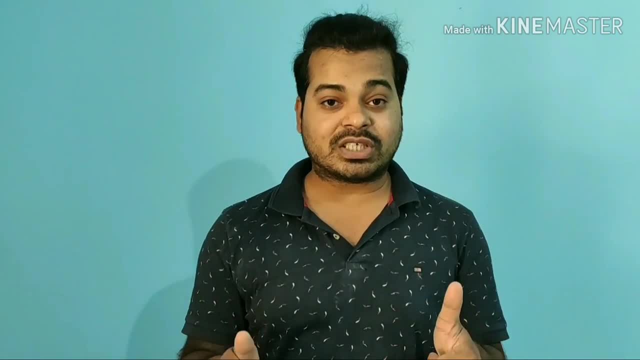 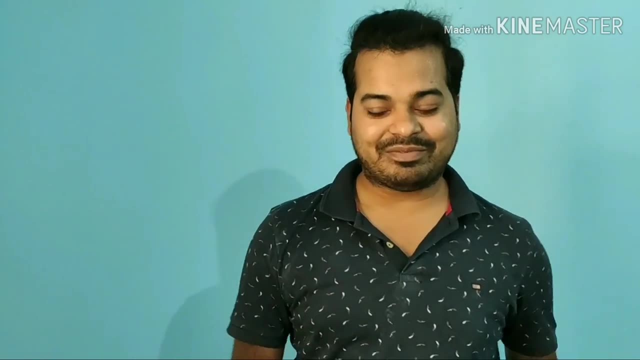 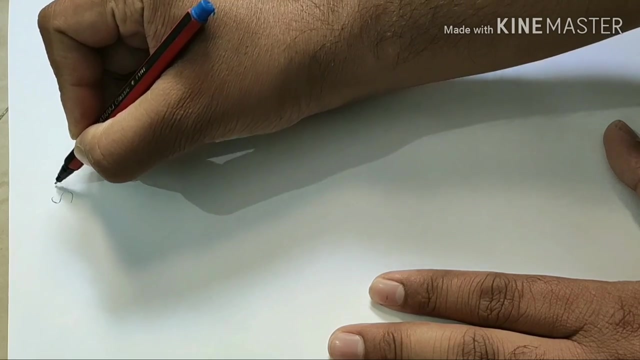 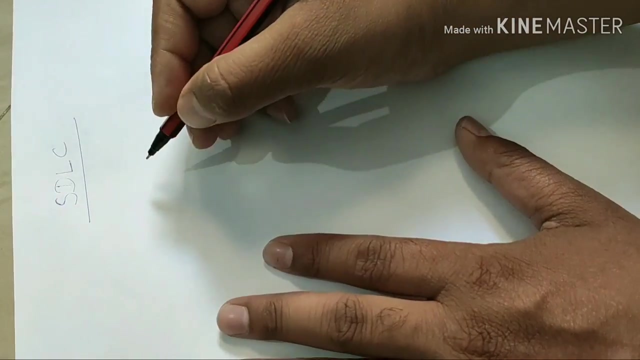 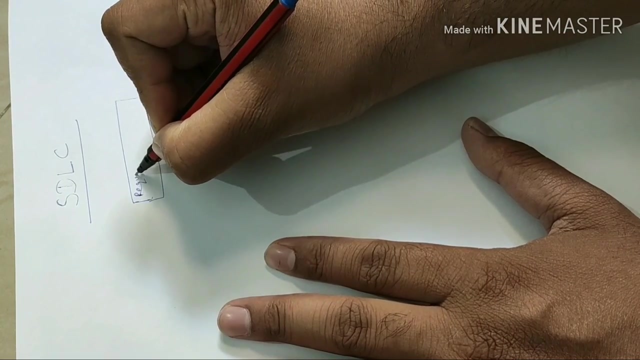 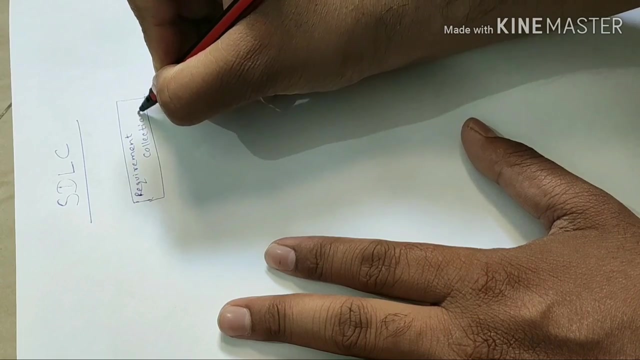 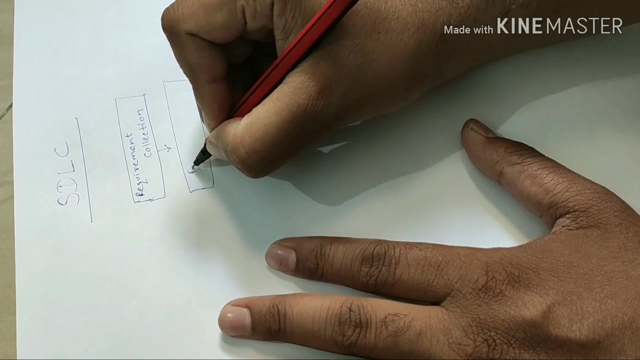 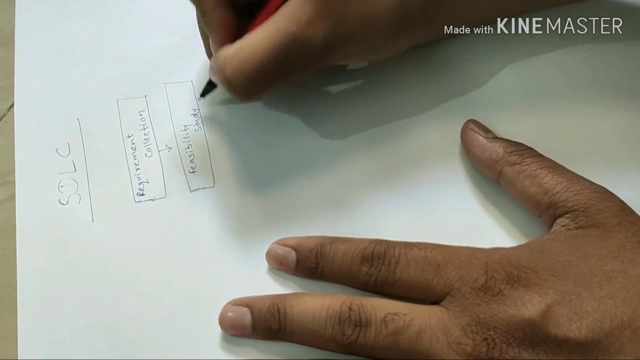 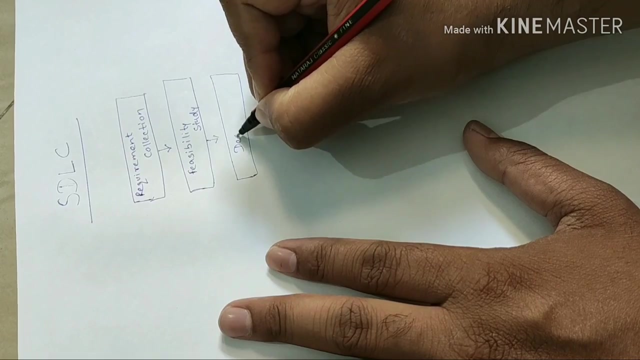 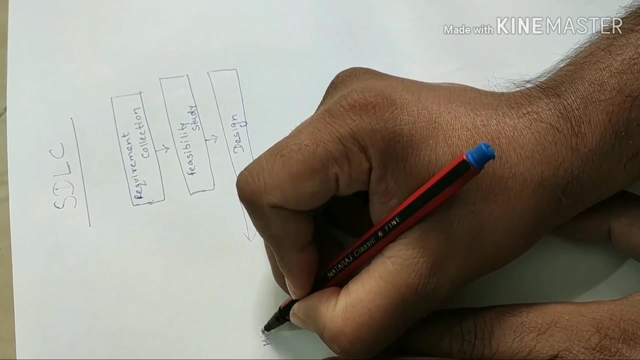 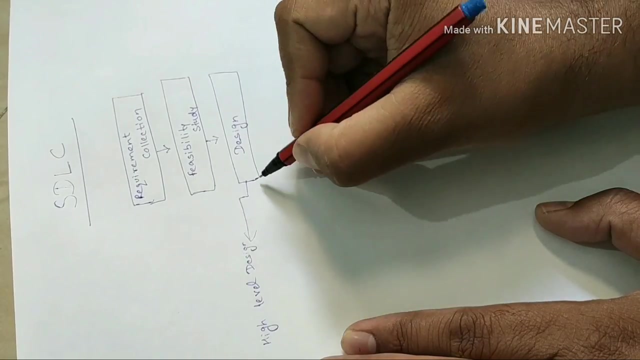 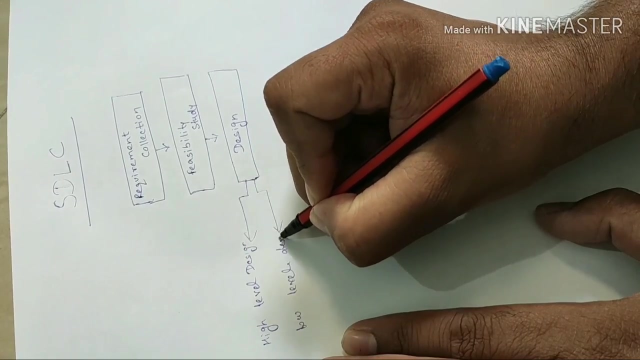 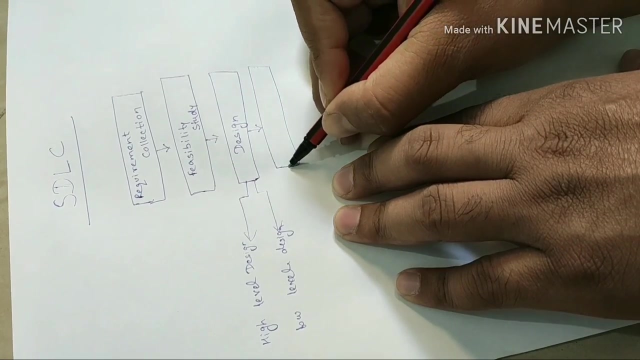 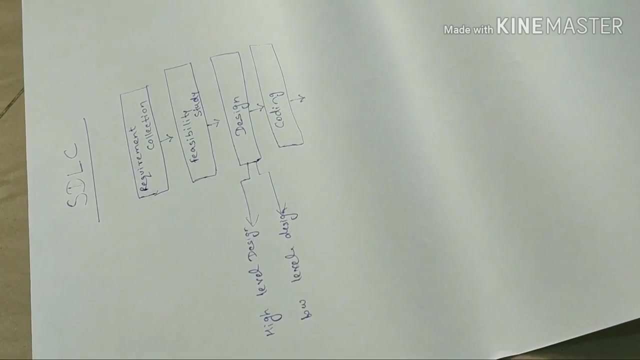 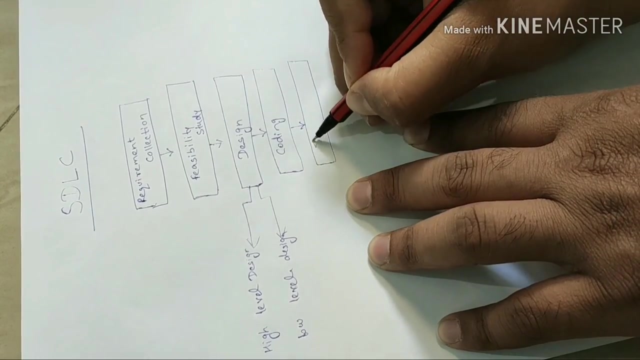 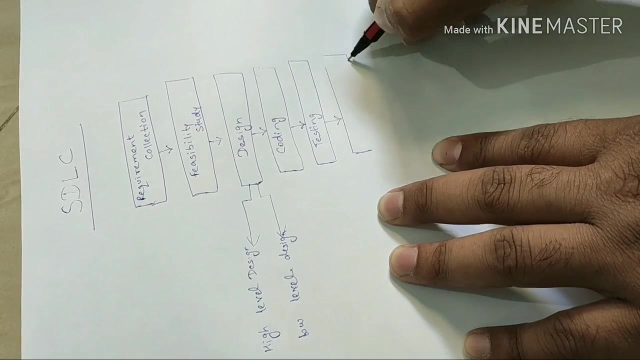 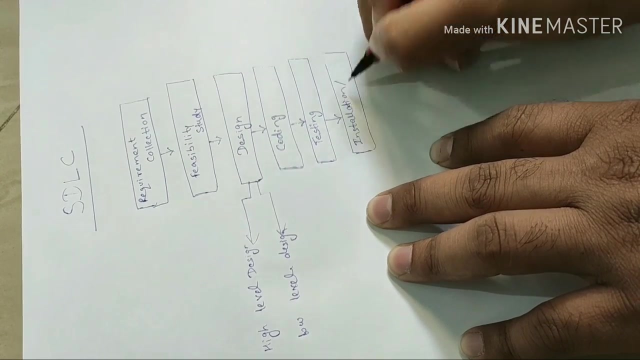 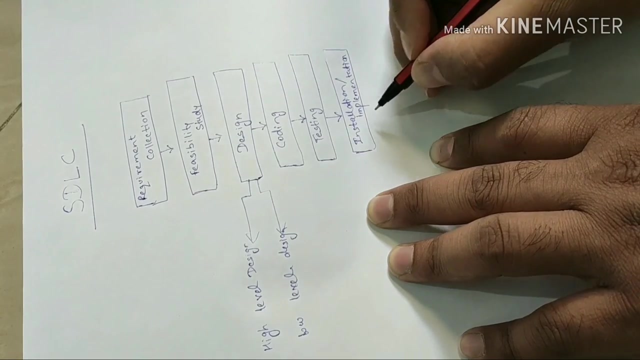 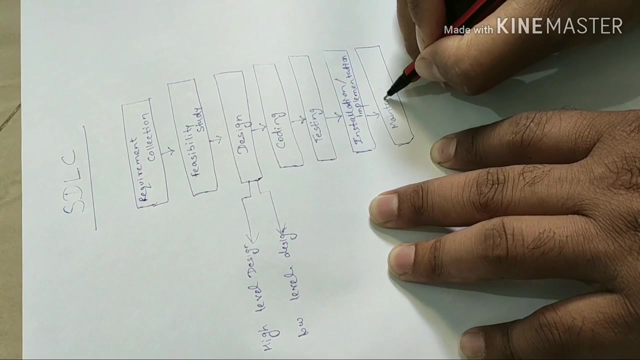 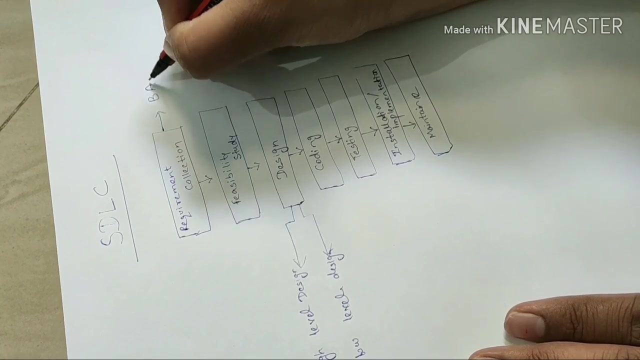 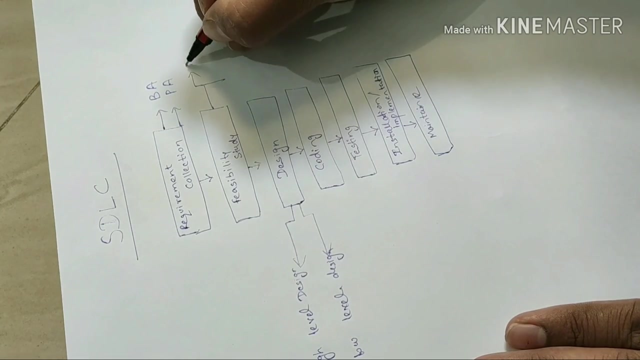 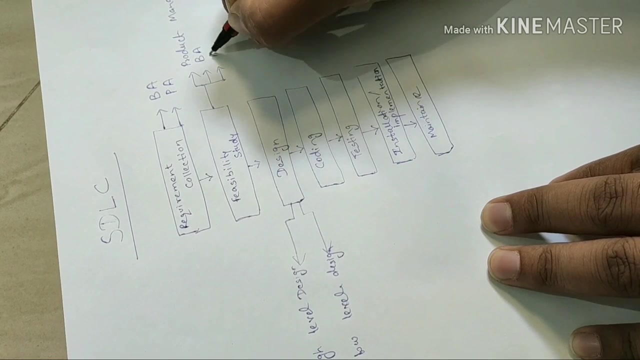